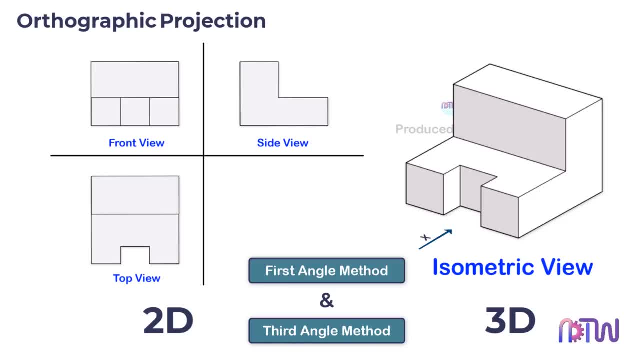 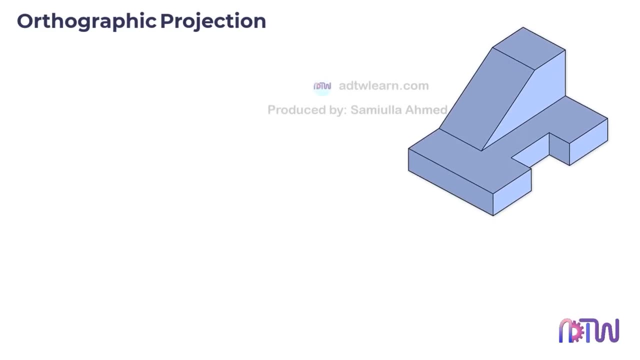 An orthographic view is a means of representing a three-dimensional view in two dimensions. It has only two axis. Let's see how we can represent this three-dimensional object in a two-dimensional view. Consider this figure Here, it is told, draw looking from the direction of X. 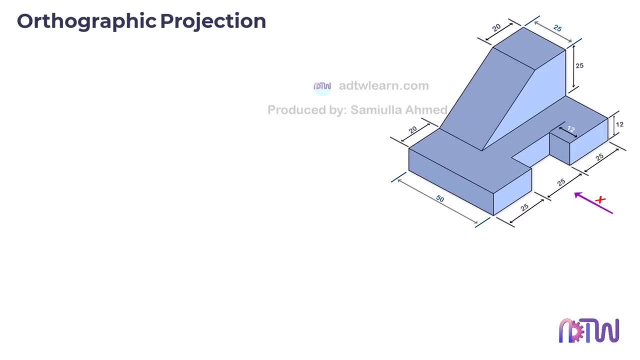 This means we should assume the viewer is viewing the object from this direction. In other words, whatever the view from this direction will be the front view of the object in the direction of X. Also in the instructions they will mention the number of views required. 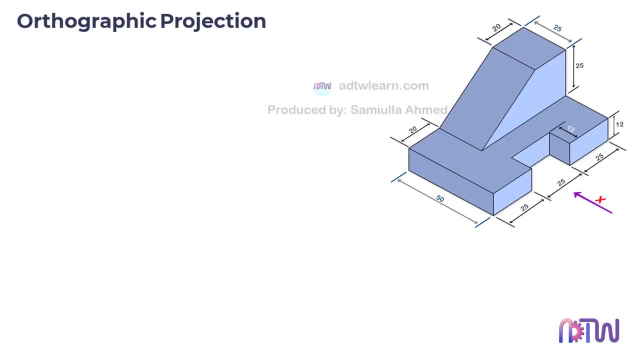 to be drawn. If it is not mentioned, then you need to draw at least three views of the object, That is, the front view, top view and side view. Also, they will mention which projection method to use, that is, the first angle or third angle method. If it is not mentioned, then you have to. 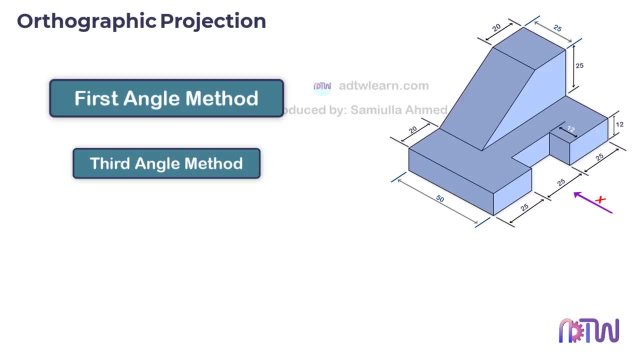 draw using the first angle method. Before starting the drawing, we need to draw the reference line, which is the XY line. We need to draw the reference line, which is the X and Y lines, Since we are following the first angle method, to draw the projection On the top, the front view. 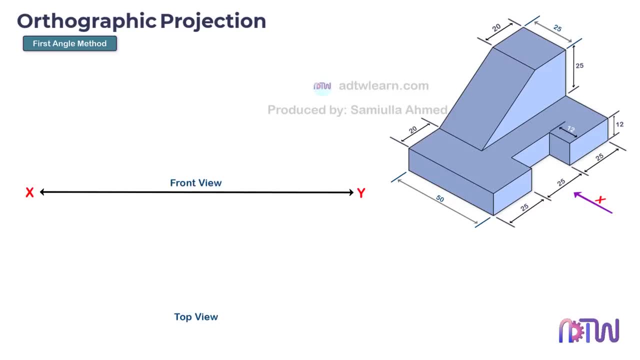 will come and, on the bottom, the top view will come. Next, we need to draw a vertical line, which we will name X1Y1.. The left side view of the object is drawn on the right side. as we are following the first angle method, Let's start drawing. 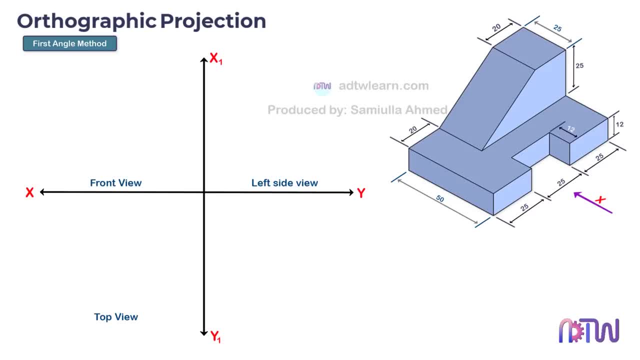 First we will draw the front view of the object, Since the direction of viewing is from this side. suppose you are standing here and looking at this object. This is how it will look. Only this part of the object is visible. Therefore, this is our front view of the. 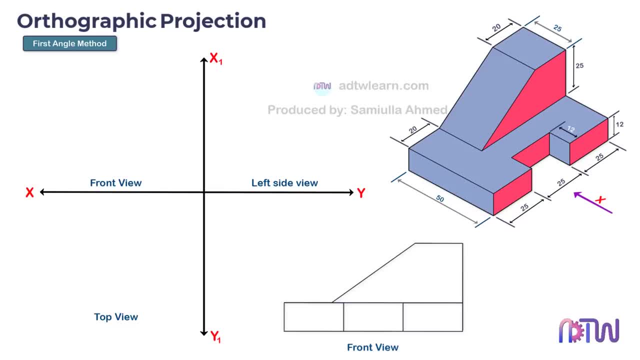 object which we need to draw above the XY line, But to do so we need the dimensions. for this view We can see. this total length is made up of three sections of 25 millimeters, which will be equal to 75 millimeters. That means this total length is 75 millimeters and these 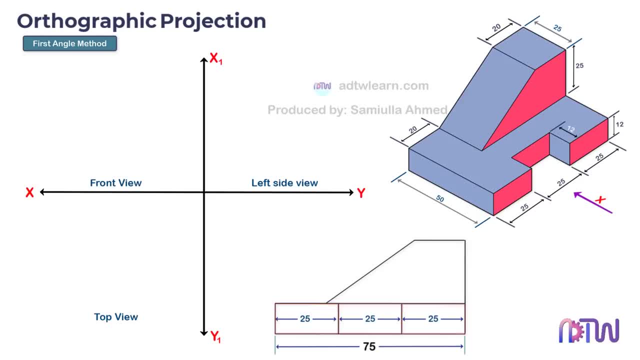 sections will be 25 millimeters each. Next, we need this height. we can see this height is given as 5 millimeters and this height is given as 25 millimeters. This width is given as 20 millimeters in the figure. And, at last, we need this width, which is given as 20 millimeters. 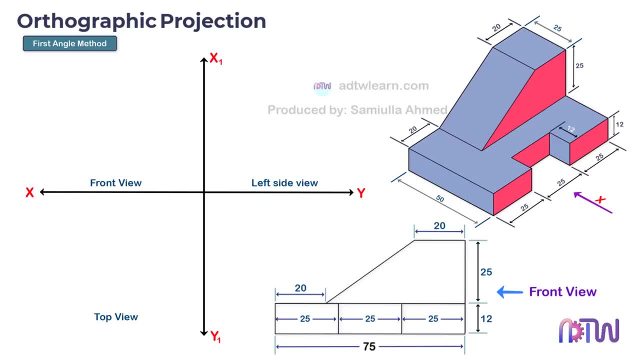 This is our front view of the object, with all the dimensions. During exams, you can draw such rough figures which will help you in drawing faster. Take a ruler and draw a horizontal line of 75 millimeters. Draw a vertical line of 12 millimeters and construct a rectangle. 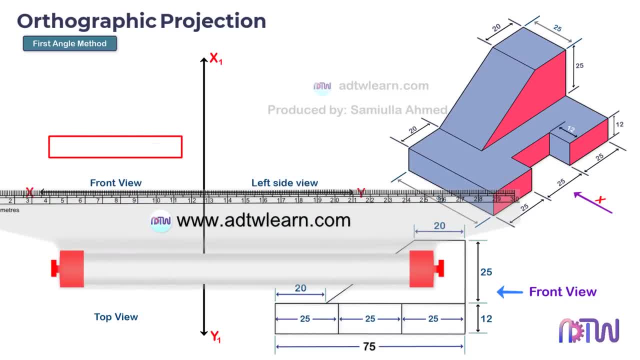 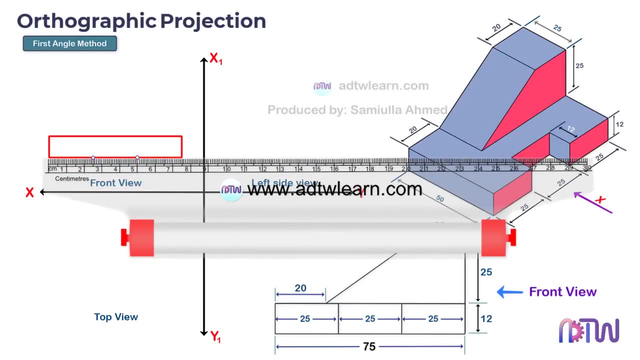 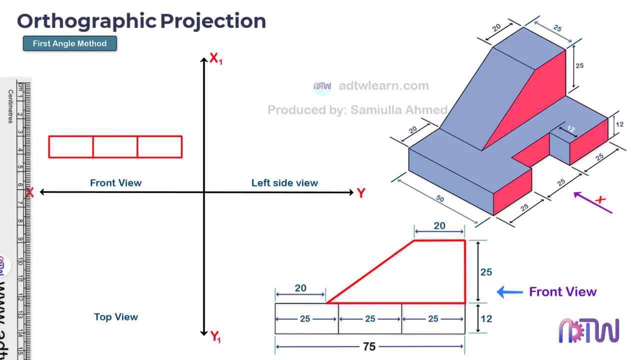 After this, we need to divide this into three parts. Take a ruler and mark 25 millimeters length and draw the horizontal lines. After this, we need to draw this section. Take a roller scale and draw a vertical line of 25 millimeters. 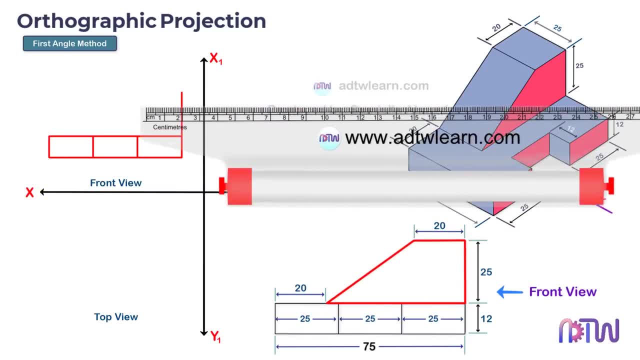 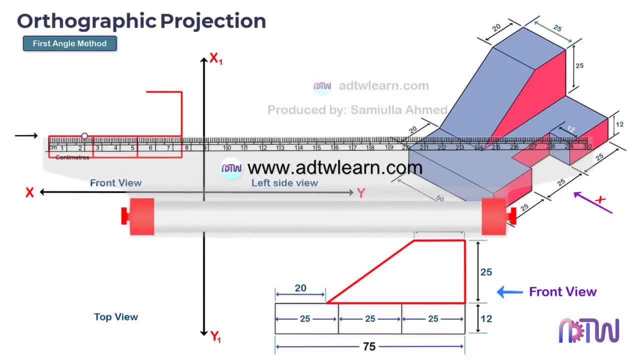 Using this line as a reference, draw a horizontal line of 20 millimeters from here. Next, using a ruler, mark a 20 millimeters length on this line from the left edge. At last, join these points with a line. This is the required front view of the object. 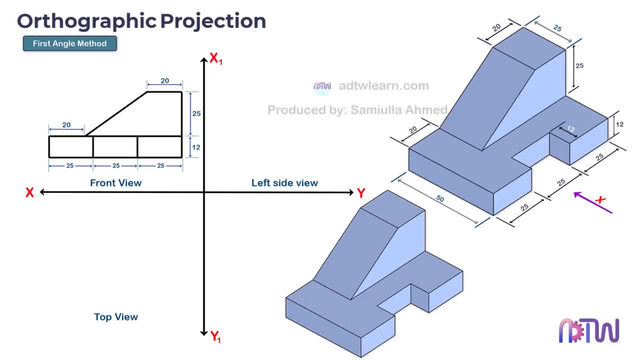 Next, we will draw the top view of this. When we view the object from the top, this is how it will look from the top. we can see only this part of the object. We already know this total length is 75 millimeters. 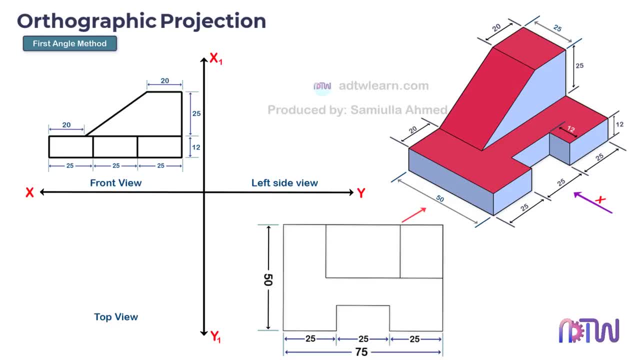 Next, this length is given as 50 millimeters, This length is given as 12 millimeters, And this rectangle's width will be 20 millimeters and its height will be 25 millimeters. This distance is given as 20 millimeters. 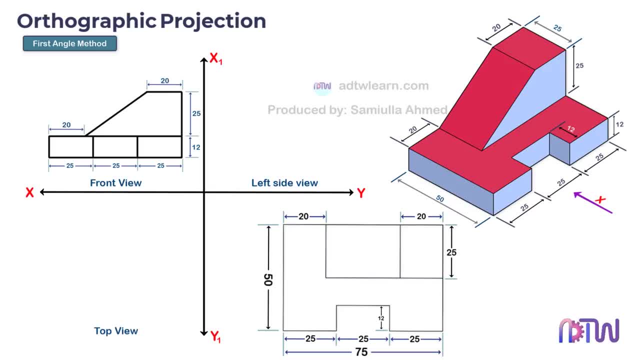 We will draw the projection lines from the front view, Then from the back view. take a ruler and draw the projection lines as shown. After this, we can use these reference lines to draw the top view. Take a ruler and draw a horizontal line. 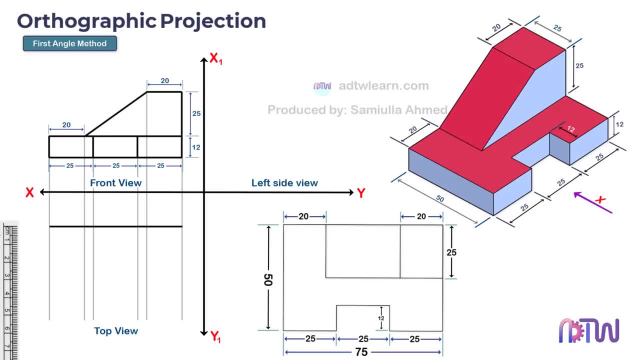 Next, draw a vertical line of 50 millimeters in length. we can see this length as 25 millimeters, which is equal to this length, which means the horizontal line will be up to this line. draw a horizontal line. this height is 12 millimeters, so from here it will be 12 millimeters up. 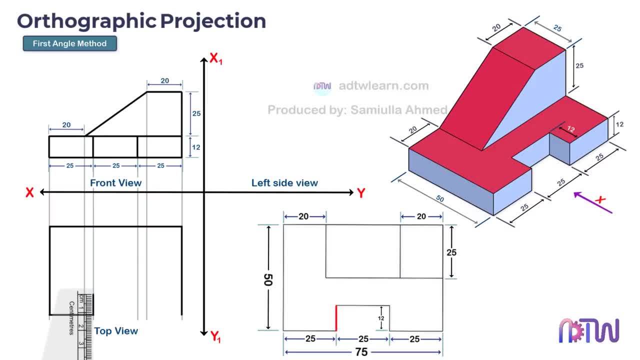 and again a 25 millimeters horizontal line, a 12 millimeters vertical line and, at last, a 25 millimeters horizontal line. next, we need to draw this section. we know this width is 20 millimeters, which is equal to this length. this height is 25 millimeters using this vertical line. 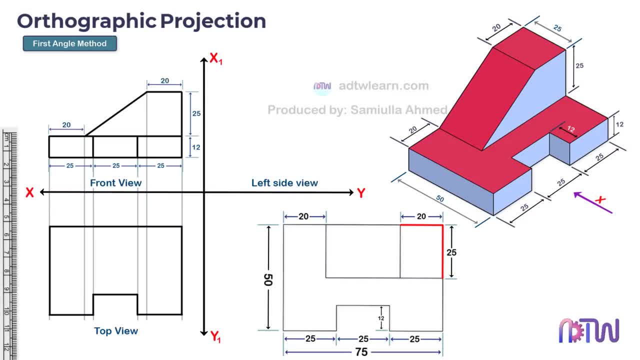 as a reference, draw a vertical line of 25 millimeters and construct a rectangle. also, we need to draw this additional rectangle which represents this inclined portion. we can see this vertical line is 25 millimeters and it is 20 millimeters away from this edge, which is equal to this length, Using the vertical line as a reference. 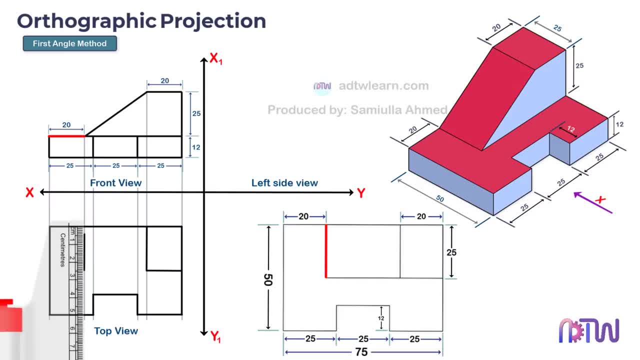 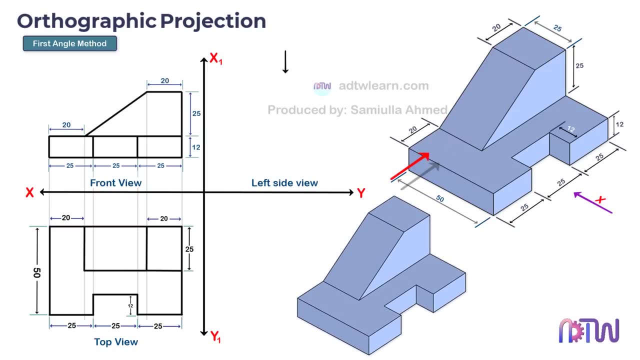 draw a vertical line of 25 mm in length. Next, take a ruler and extend this horizontal line up to this line. This is the required top view of the object. At last, we need to draw the left side view of the object here. When we see the object from the left side, this is how it will. 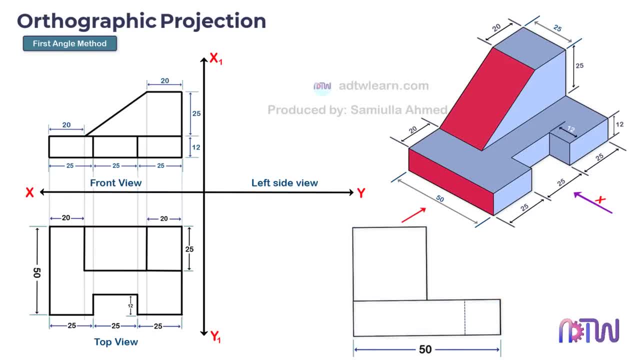 look, We know this length is 50 mm and we can see this height is 12 mm. Next, this height is given as 25 mm and this width is 25 mm. We got all the required dimensions for the side view. 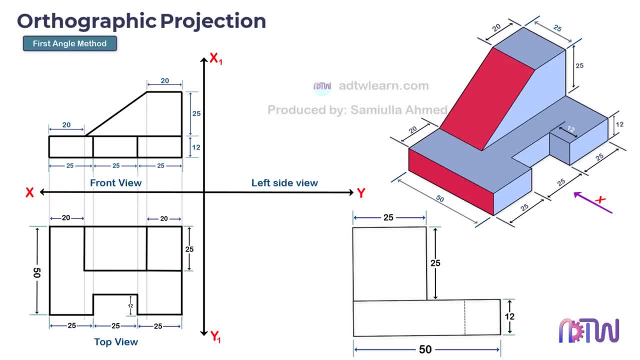 First we will draw the horizontal projection lines from the front view of the object. Also, we can draw the projection lines from the top view. To do so, first draw an inclined line which will be at 45 degrees. After this, draw the projection lines from the top view, Extend these lines up to this inclined line. 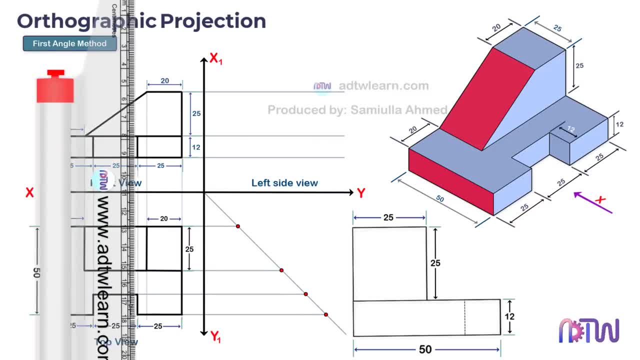 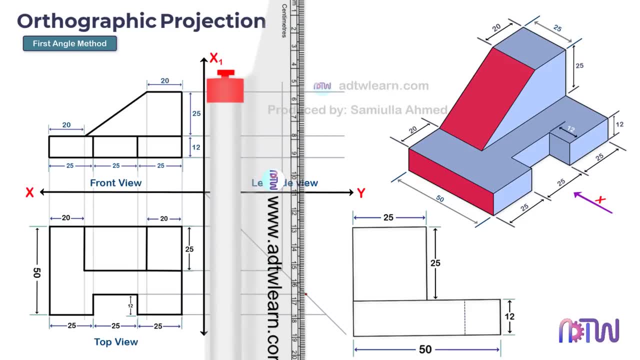 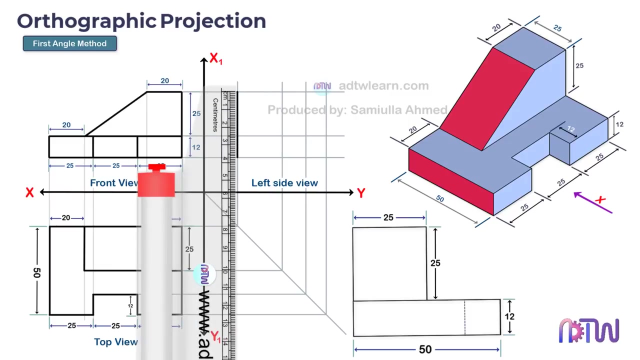 And draw the vertical lines from each of these intersection points. These lines will help us in drawing the side view. Take a roller scale and draw a vertical line of 37 mm in length. After this, draw a horizontal line of 50 mm in length, as shown. 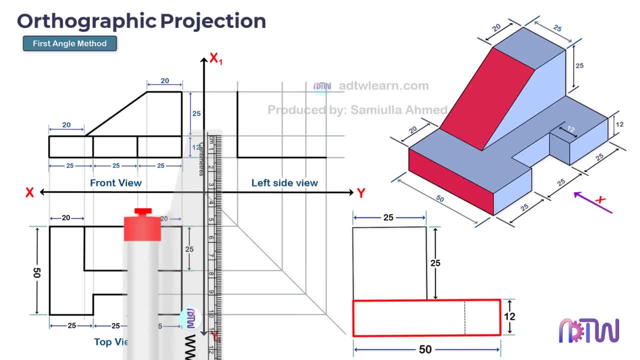 We need to construct this rectangle. We can see its height as 12 mm. Draw a vertical line of 12 mm and construct a rectangle. Next, we need to construct this shape. We can see its height as 12 mm. Next, we need to construct this shape. We can see its height as 12 mm.